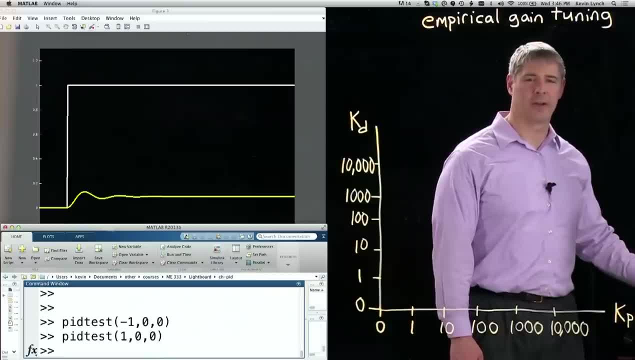 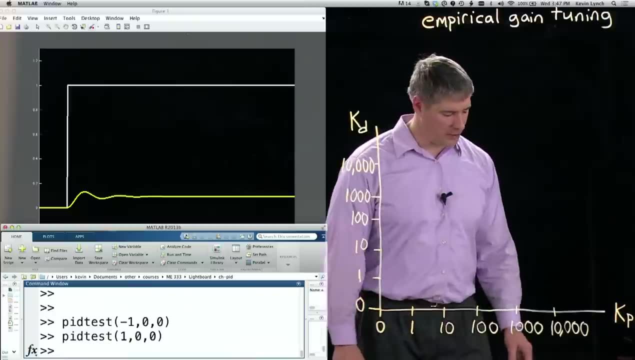 Gain and zero, and zero for the integral and derivative, And now we can see that the output rises closer to the reference value, But it's still not doing very well. So this is my first guess. I'm going to mark that with a one. 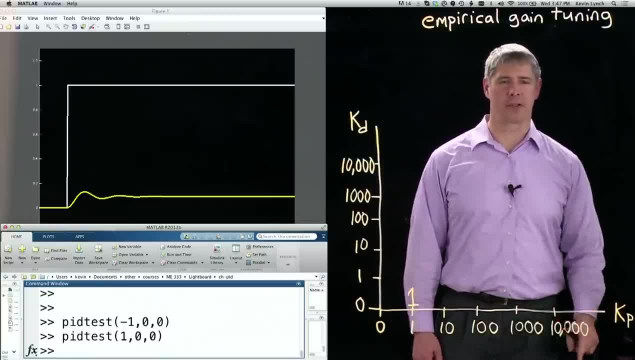 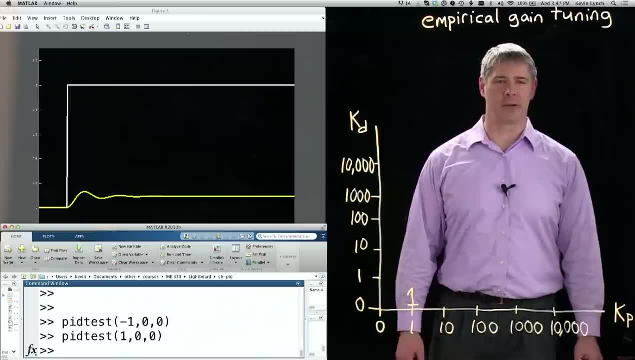 So this is my K sub P axis for proportional gains, K sub D for derivative gains, And my first guess here was at K sub P equal to one, K sub D equal to zero, And I'm still far away from my desired value. 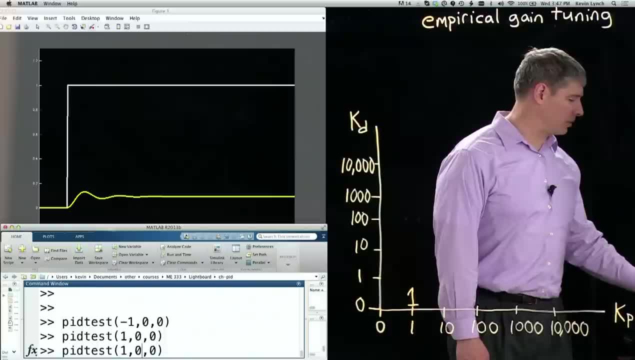 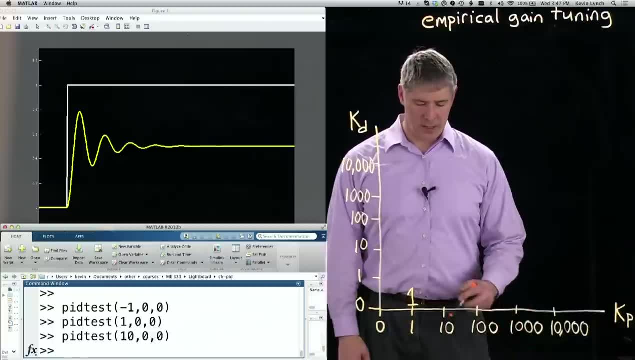 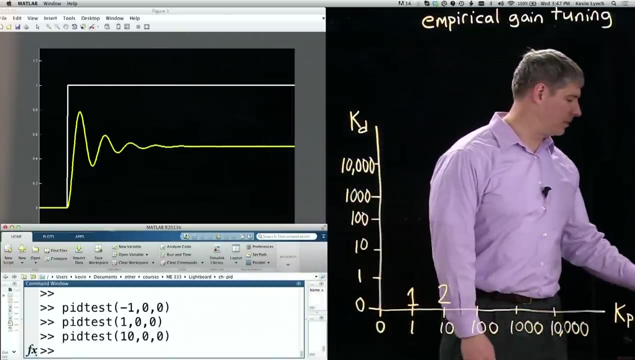 I need to increase my proportional gain. So let me raise it to ten, And now you can see that we're coming closer to the desired value. So this is my guess number two, But we're still pretty far away. Let's try increasing it by another factor of ten. 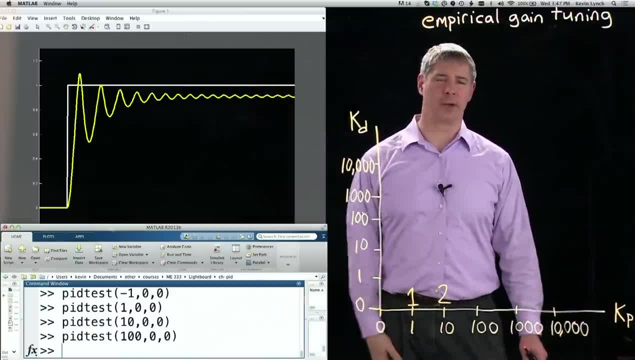 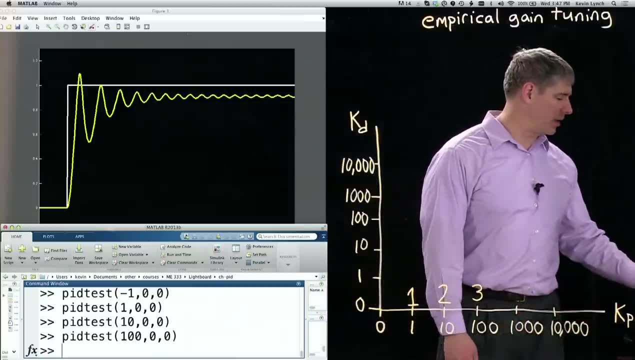 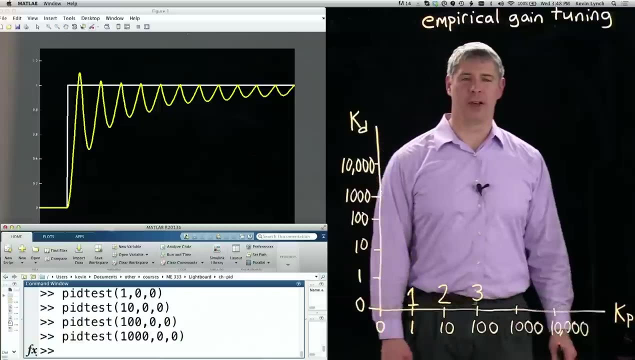 Okay, now we're getting closer, But we still have a lot of ringing and overshoot here. So let me mark this as guess three. For the heck of it, let's try increasing the gain by another factor of ten. Okay, and now we're not getting any improvement in behavior. 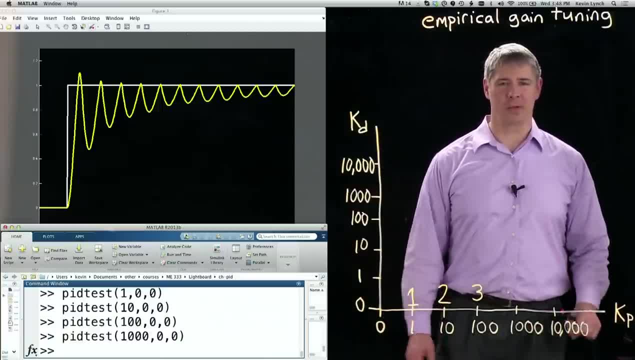 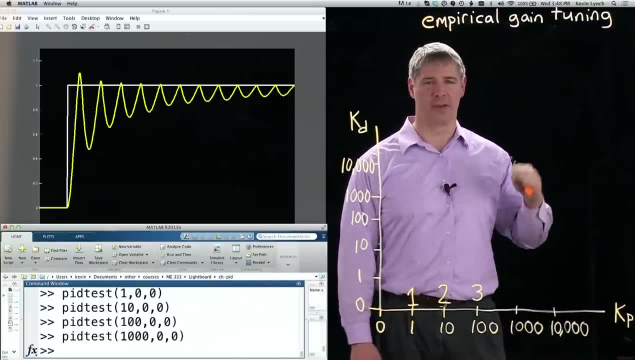 In fact, if we took a look at our control signal, we would see that because we have such large gains for K sub P that the control signal is always saturating, It's always at its maximum or minimum limit, So we're getting this kind of strange-looking behavior here. 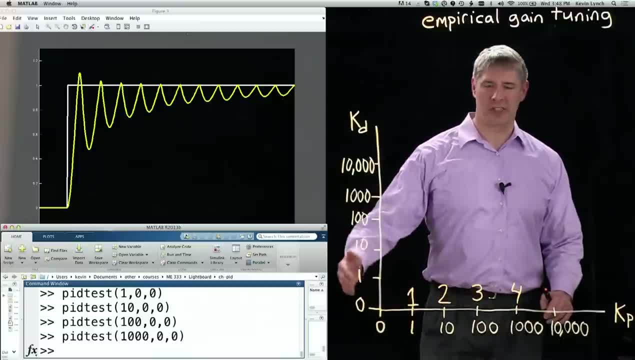 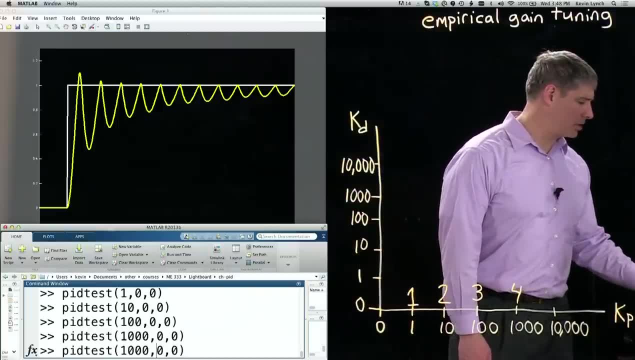 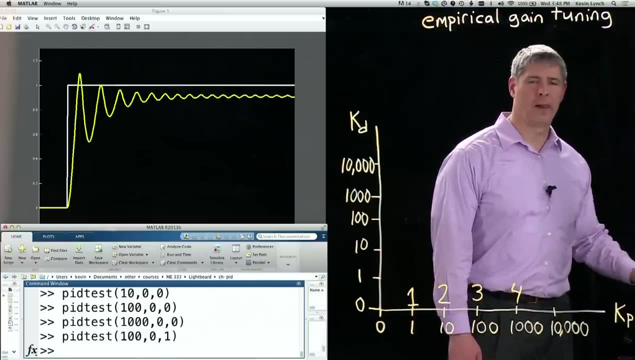 And that says we've probably gone too far Just in the K sub P direction. So let's backtrack a little bit and try adding some damping. So we'll reduce our proportional gain to a hundred, Make the derivative gain one, And I see that there's not much of an effect. 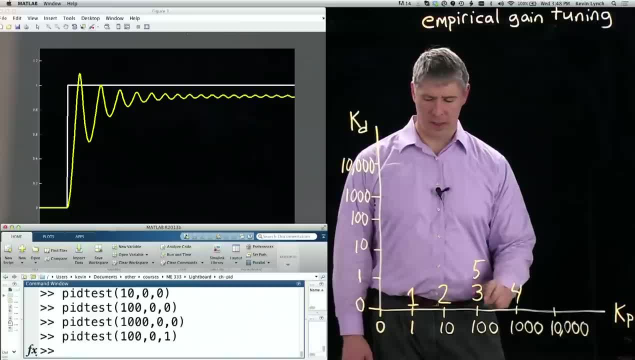 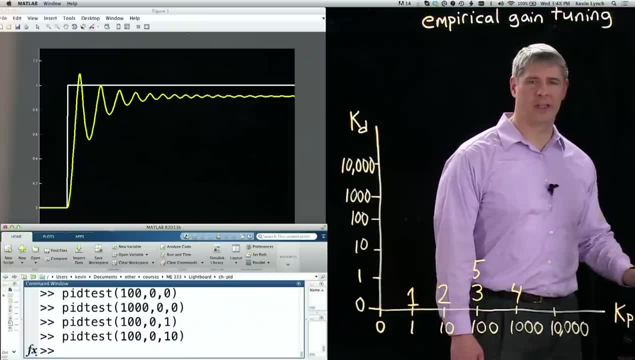 So this is guess number five. Let's try increasing that by a factor of ten. So we're going to increase the derivative gain by a factor of ten. You can see it damps out. It damps out a little bit, but still not very much. 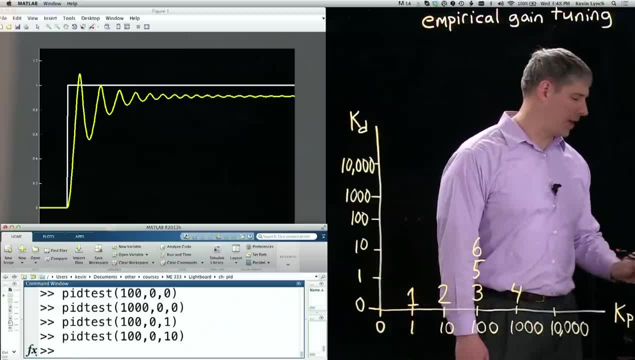 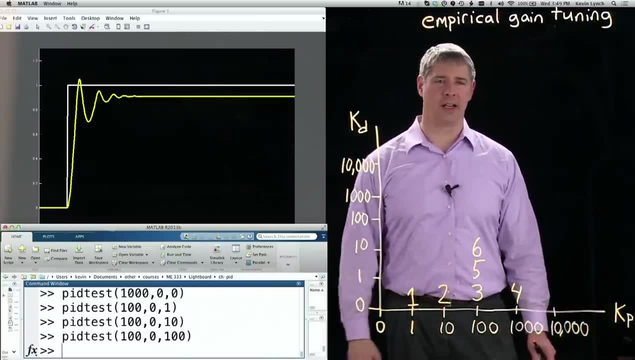 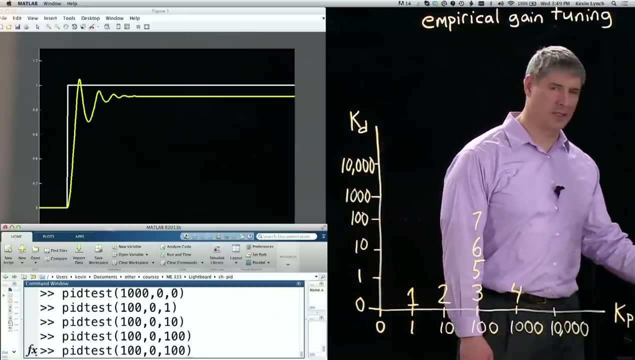 We're getting a lot of oscillation and overshoot. Let's increase by another factor of ten. Okay, now we're starting to see more damping. It's still oscillating a little bit, So that's up here. Let's try increasing the damping by another factor of ten. 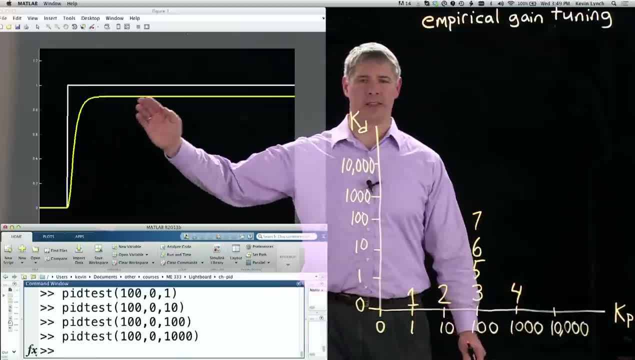 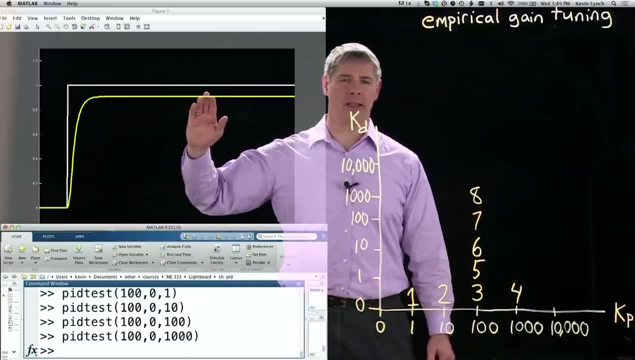 Okay, now we're getting something that looks pretty good. So we're getting this smooth rise and settling. So this is guess number eight. So this response doesn't look bad. We still have some steady state error. Let's try increasing the stiffness and increasing the damping together. 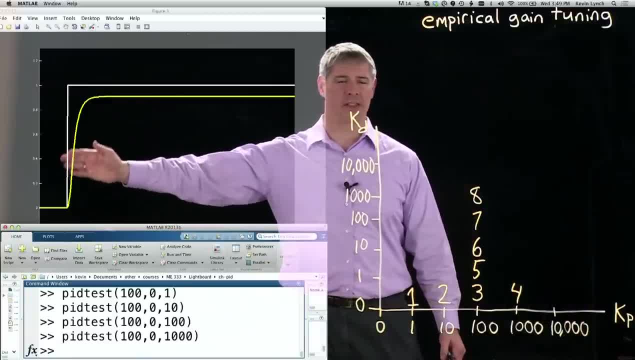 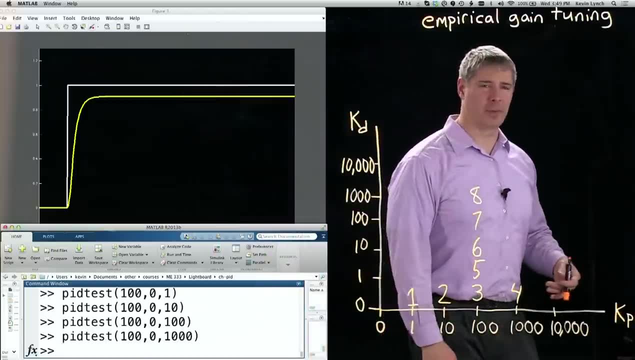 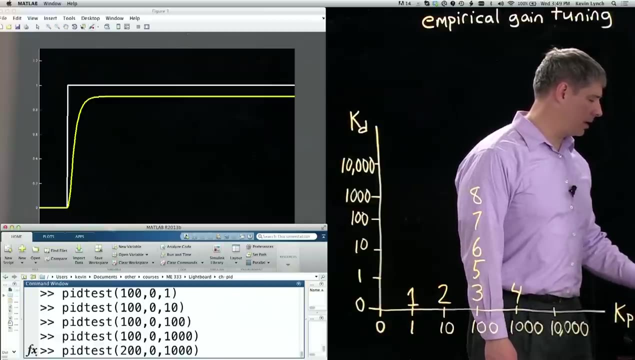 Hopefully thereby keeping the good shape of our response- And this is called the transient response- While hopefully reducing this steady state error. So I'm going to double both the proportional and the derivative gain. So K sub P is two hundred, K sub D is two thousand. 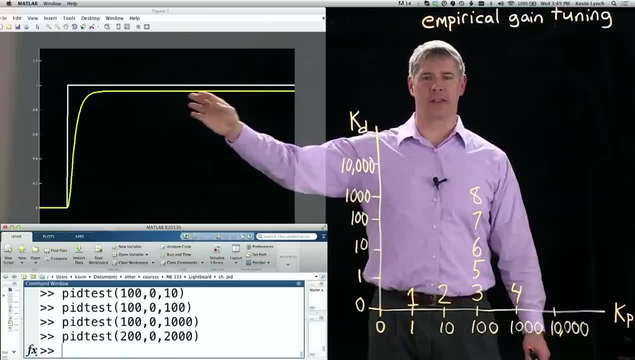 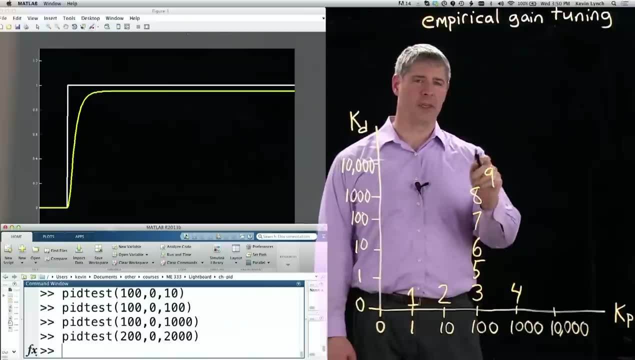 Okay, now I'm getting even better performance. Still the good transient response, Less steady state error. So this is guess number nine. We've increased in both K sub P and K sub D. So let's stop there with our PD gain tuning. 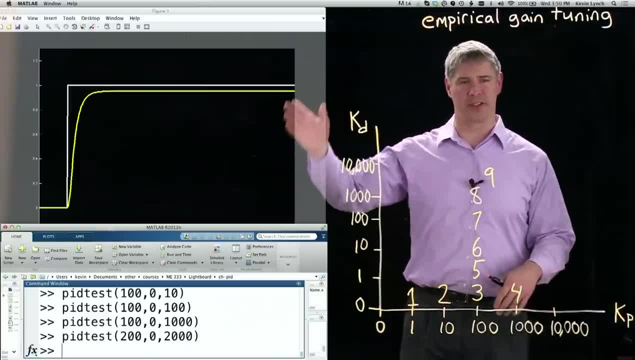 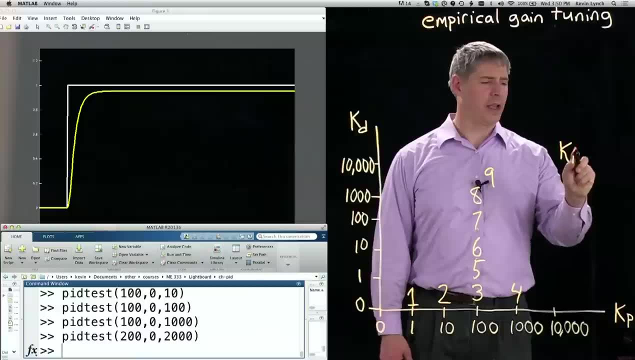 And, by the way, we can't make our gains arbitrarily high, or else we're going to see chattering behavior. Now let's try adding a little bit of integral action. So let's start out with K. I is equal to one, So keep P and D as that. 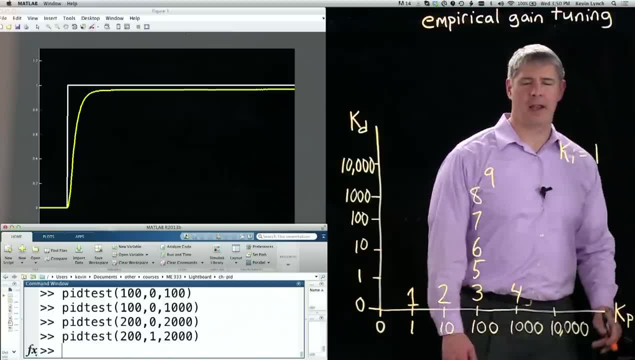 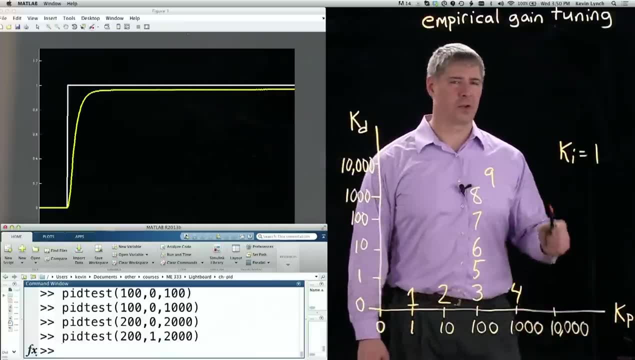 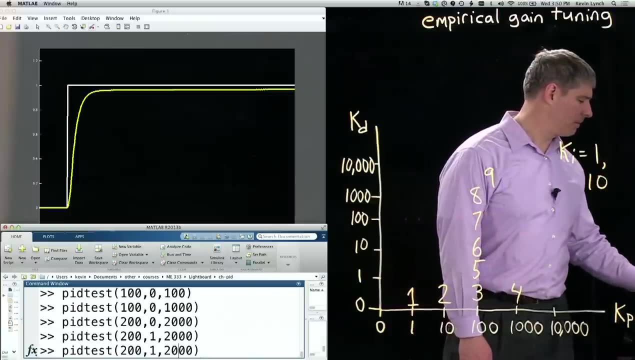 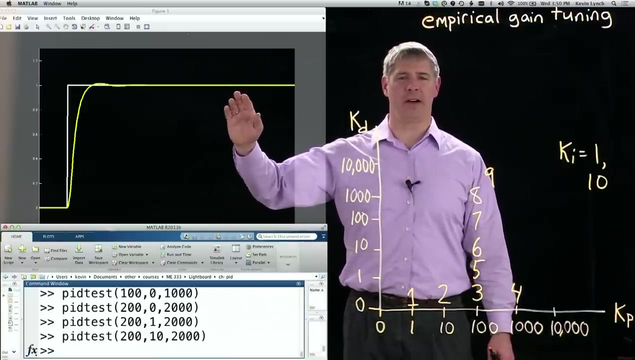 There they are And if you notice here now, the response starts slowly heading towards the desired steady state value. So we're seeing some effect of that. K sub I, Let's increase by a factor of ten. Okay, now we're seeing that we're getting essentially zero steady state error. 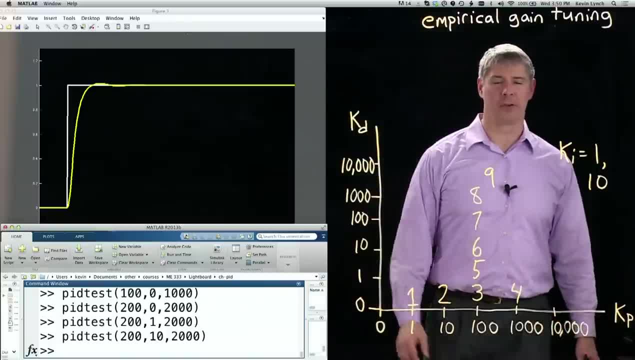 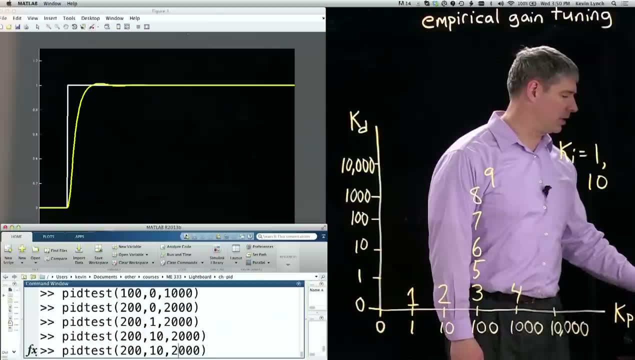 But we've introduced a little bit of overshoot, And that's what integral gain will do. It tries to reduce steady state error. It may induce some instability And if we wanted to emphasize that, we could increase that gain to 100. 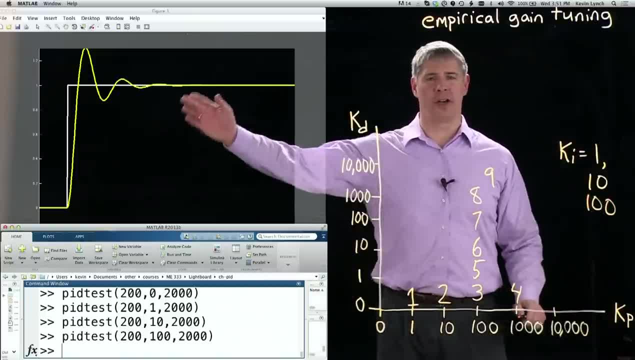 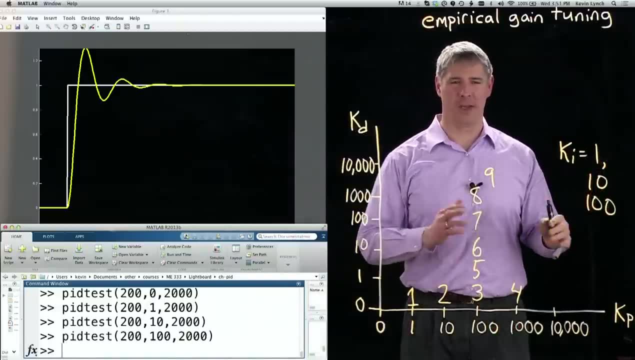 And now you're seeing lots of overshoot and oscillation. So we've gone too far with K sub I. So if we go back here, it looked like one was pretty good, It looked like ten was pretty good, But maybe somewhere in between.